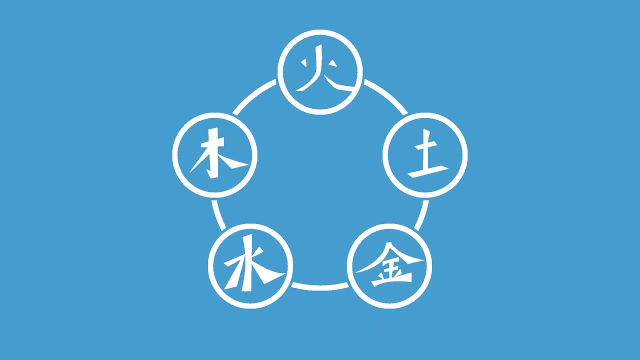 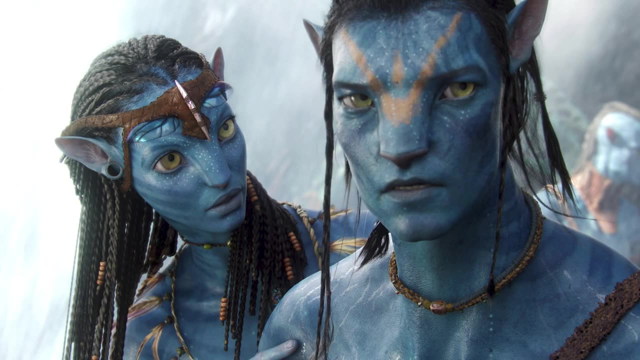 Five. It's a powerful number, isn't it? The five East Asian elements, the five Olympic rings, or even, in the fictional world, the Scooby gang, the Power Rangers or the Avatar gang? No, not the blue ones, these guys. As time marches on and technology advances, we have a new collection. 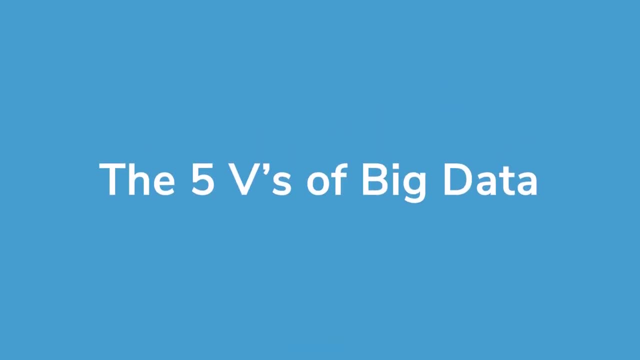 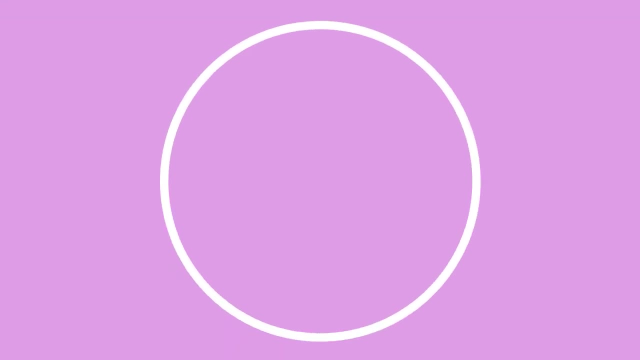 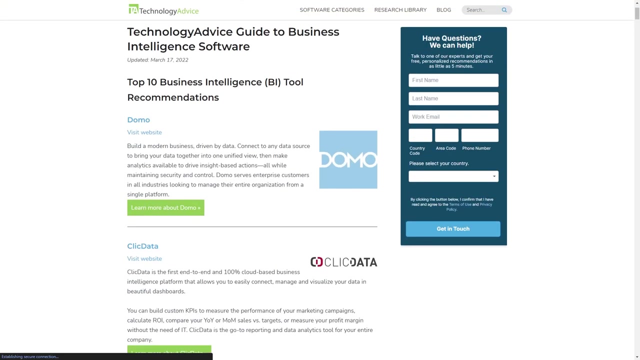 of five to look towards The five Vs of big data: Volume, velocity, variety, veracity and value. Before we get into all that, though, hi, I'm Kyle, and today I'll be chatting with you about those five Vs of big data, And if you want more info on business intelligence tools to help your 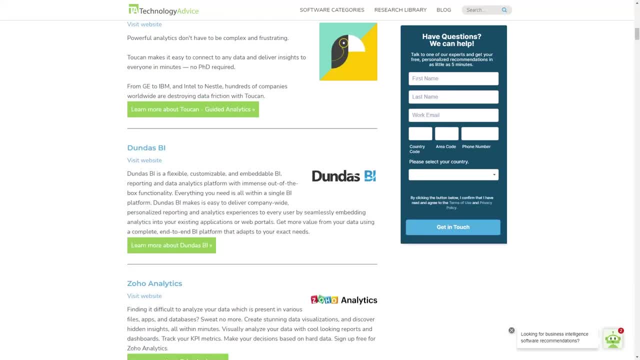 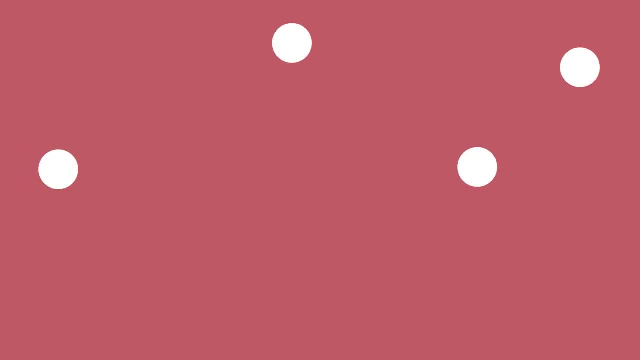 company navigate big data. check out our website at technologyadvicecom If you find this video useful. it'd help me a lot if you hit those like and subscribe buttons down below. While big data- the trillions of data points collected across organizations- can be mined for useful info. 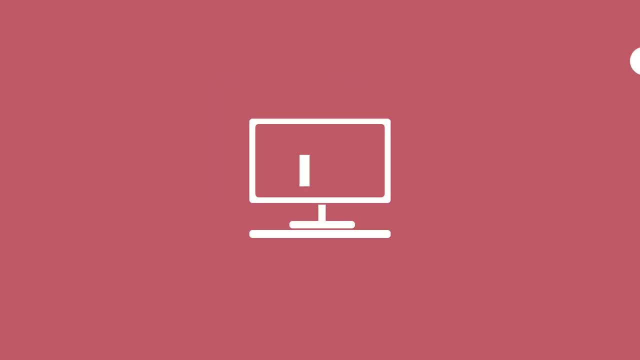 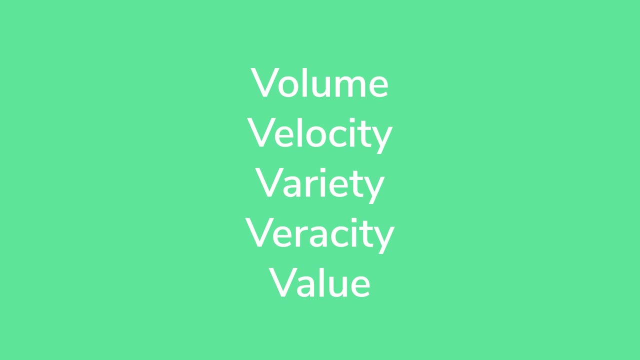 it's how the data is analyzed and what those organizations do with that insight. that's important. There are numerous challenges, namely those five Vs I mentioned earlier, that all organizations have to tackle when it comes to working with big data. Volume refers to the colossal amount of data. 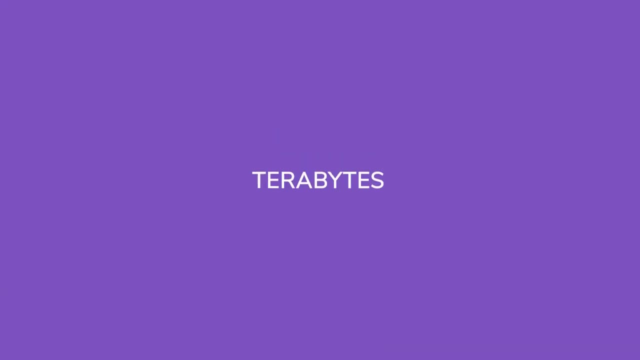 that inundates organizations. Companies of 15 years ago handled terabytes of data. Today, data has grown to petabytes, if not exabytes of bytes, That's 1,000 to 1 million terabytes that come from sources such as transaction processing systems, emails, social networks. 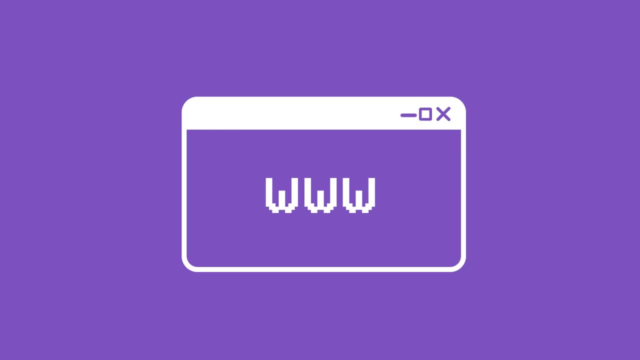 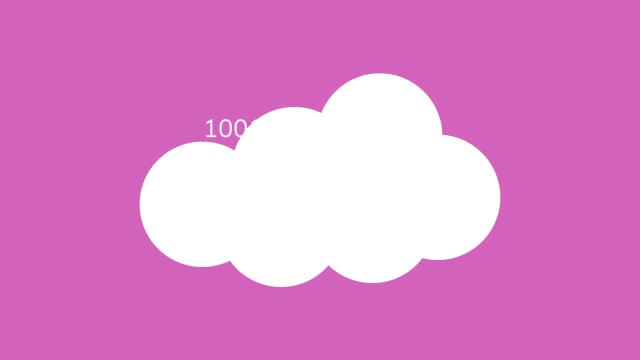 customer databases, website lead captures, monitoring devices and mobile apps To handle all of this. data managers use data to manage their data. They use data to manage their data Data lakes and warehouses or data management systems. They store it on clouds or use service. 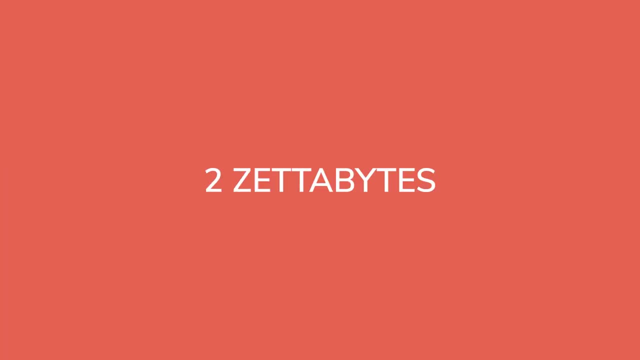 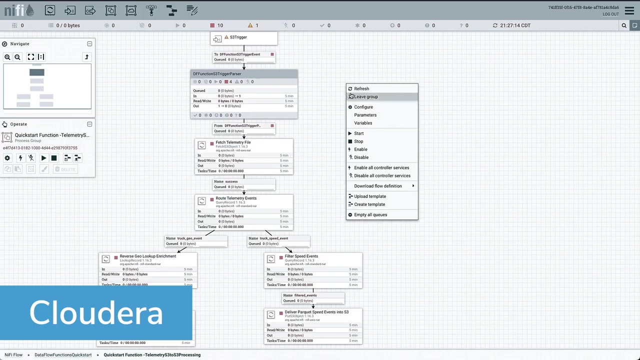 providers such as Google Cloud, And as global data grows from two zetabytes- that's, 1 billion terabytes each at the beginning of the decade- to 181 zetabytes a day by 2025,, even these may be insufficient. Apache's Hadoop splits big data into chunks, saving it across clusters of servers. 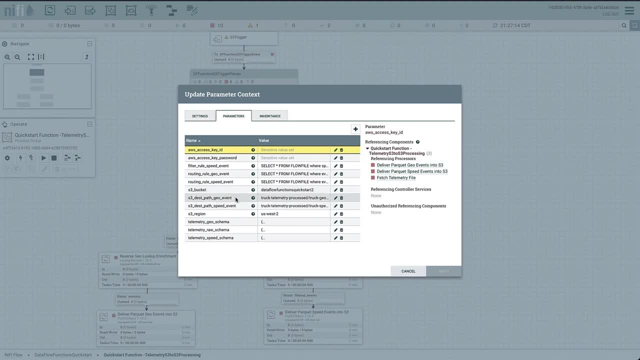 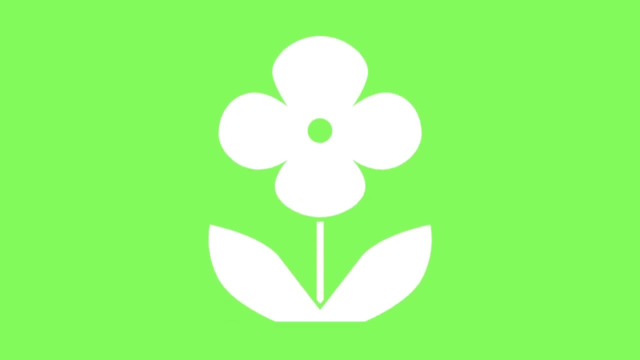 Check out Cloudera Enterprise 4.0 with its high availability features, making Java-encoded Hadoop more secure. Big data grows fast. Consider that, according to Zetasphere, there are over 3,400,000 emails, 4,595 SMS, 740,741 WhatsApp messages and almost. 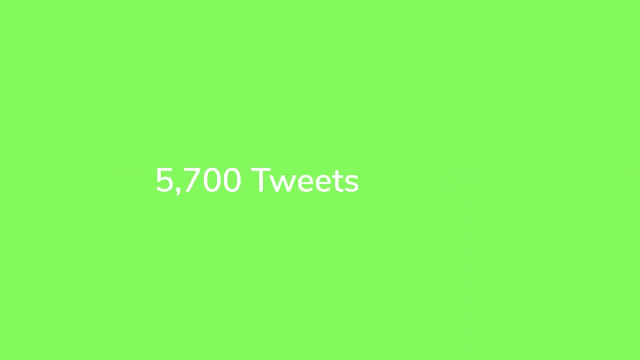 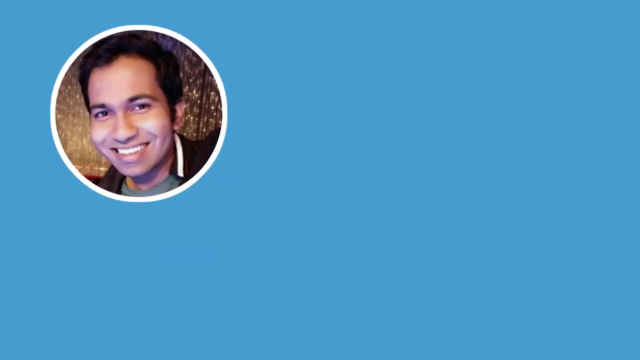 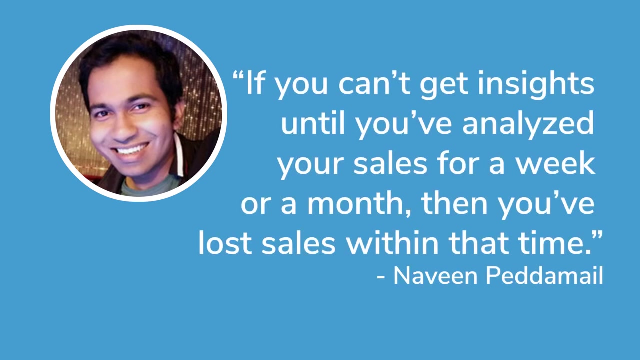 69,000 Google searches, 55,000 Facebook posts and 5,700 tweets made per minute. More critical still, data ages fast. As Walmart's former senior statistical analyst, Naveen Petimale, said, if you can't get insights until you've analyzed your sales for a week or a month, 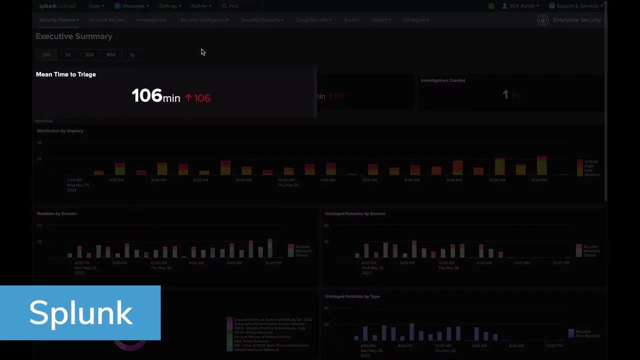 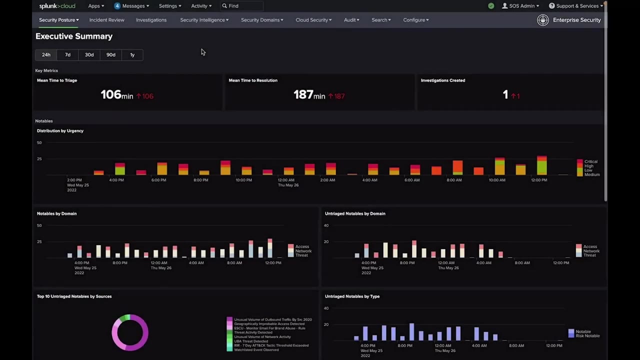 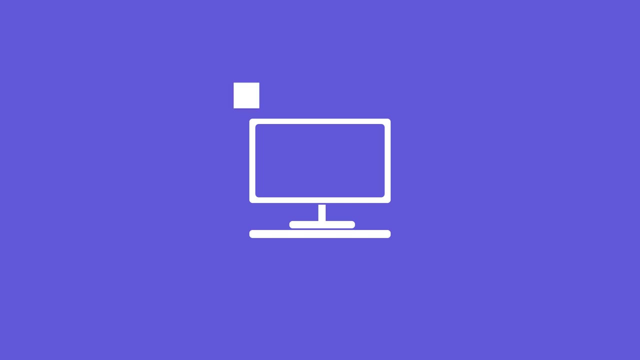 then you've lost sales within that time. Competitive companies need some capable business intelligence tools to make timely decisions. For instance, Splunk Enterprise monitors operational flows in real time, helping business leaders make timely decisions. That said, it is expensive for large data volumes. Variety refers to the different types of 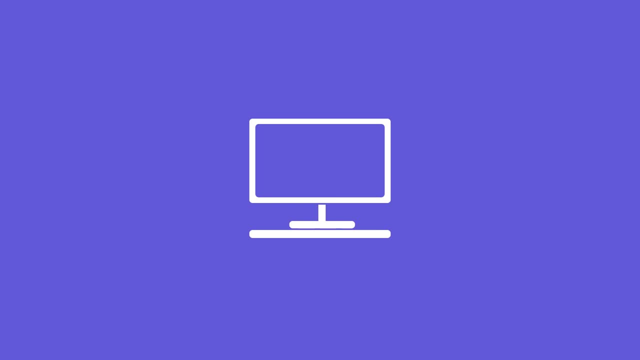 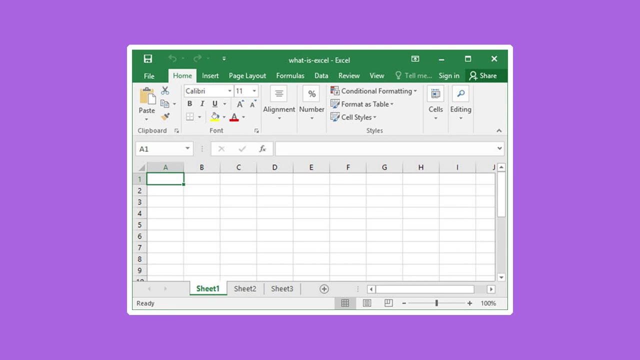 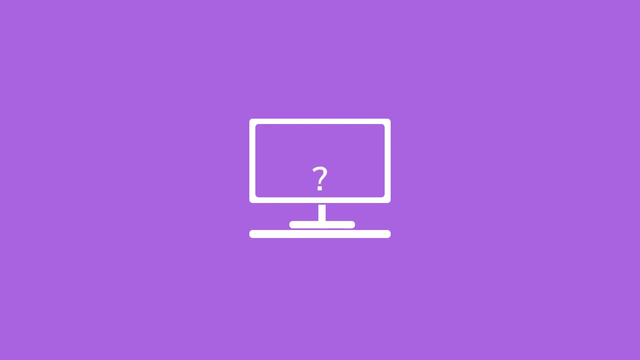 digitized data that inundate organizations and how to process and mine these various types of data for insights At one time or in the future. it's going to be a lot more expensive. Today you also have unstructured information that evades management and comes in diverse forms. 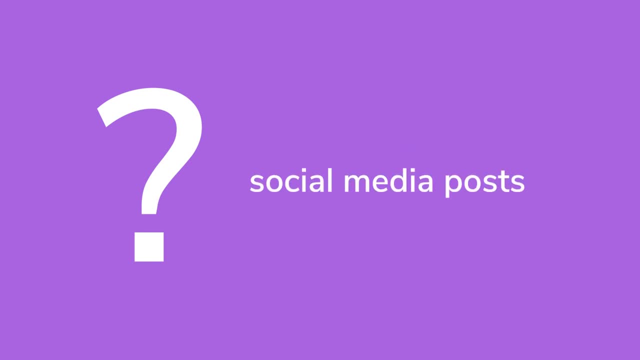 such as emails, customer comments, SMS, social media posts, sensor data, audio, images and video. Companies struggle with digesting, processing and analyzing this type of data, and doing so in real time. For small to mid-sized companies, Tableau is ideal, since it is also. 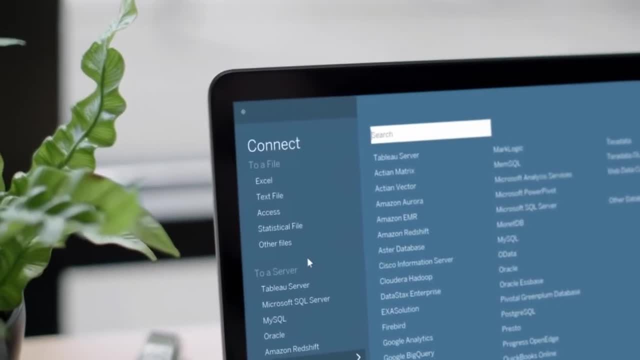 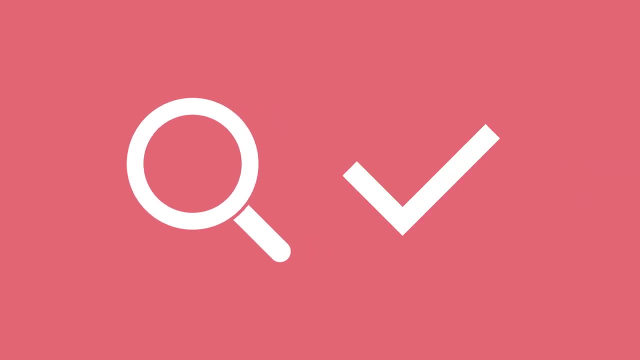 designed for non-technical users and helps to analyze and analyze data in real time. Veracity is arguably the most important factor of all of the five Vs, because it serves as the premise for business success. You can only generate business profit and impact change with thorough and correct information. Data can only help organizations if it's clean. 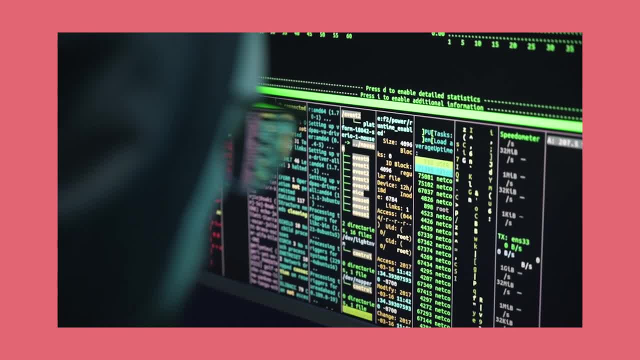 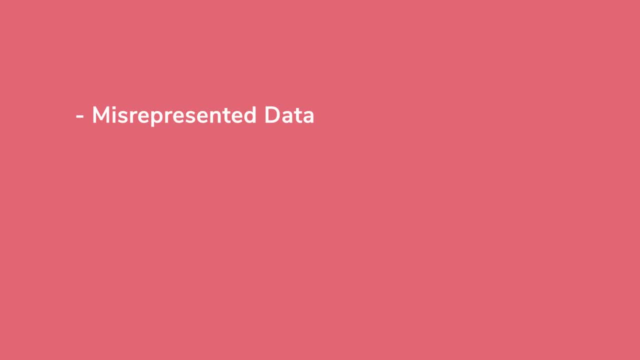 That's, if it's accurate, error-free, reliable, consistent, bias-free and complete. Contaminating factors include statistical data that misrepresents the information of a particular market, Meaningless information that creates a lot of confusion and confusion. The data that creates confusion and confusion is the data that creeps into and distorts the data. 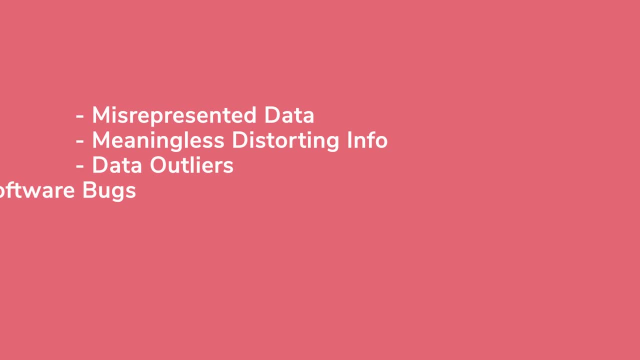 Outliers in the data set that make it deviate from the normal behavior. Bugs in software that produce distorted information. Software vulnerabilities that could cause bad actors to hack into and hijack data. Human agents that make mistakes in reading, processing or analyzing data, resulting in incorrect information. 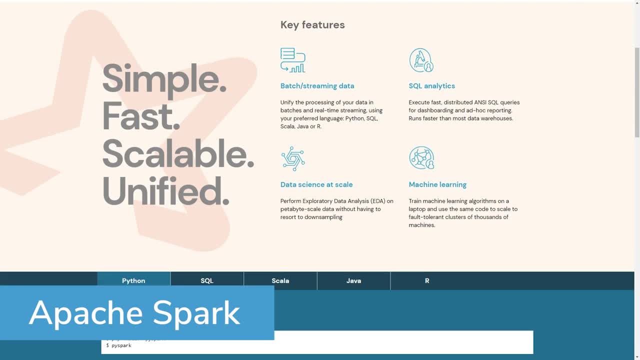 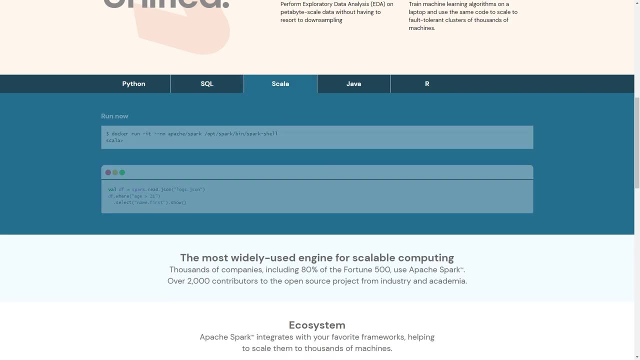 To tackle this. a BI system must be able to handle queries to check the veracity of the data that passes through the system, Multilingual and scalable. Apache Spark is good for quick queries across data sizes. Data is the new competitive advantage, but that's only if you convert your information.